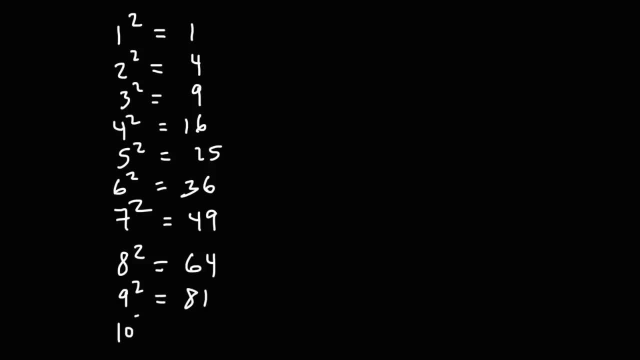 9 squared is 81.. 10 squared is 16.. Now I'm going to continue. 16 squared is 366.. 17 squared is 289.. Next we have 19 squared, which is 361.. And finally, 20 squared is 400.. 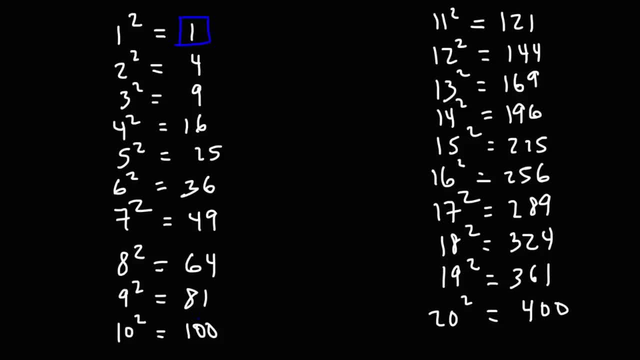 So notice that these two numbers are the same. So anytime you square a square, you're going to get a square. So if you have a square number that ends in a 1 or a 9, the perfect square will have a 1 as the unit digit. 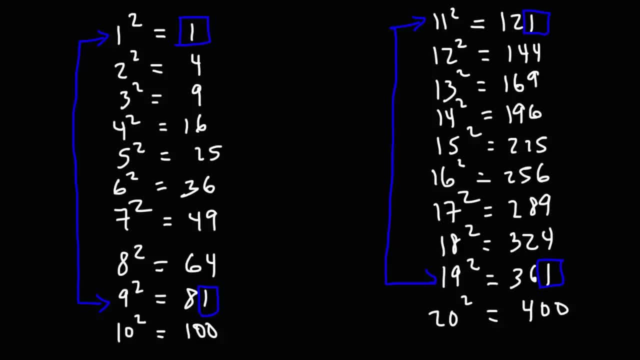 You can see that here as well. Next, we have 4.. Anytime you square a number with a 2 or an 8, the perfect square will end in a 4.. Next, it ends in a 4. And it's 9.. 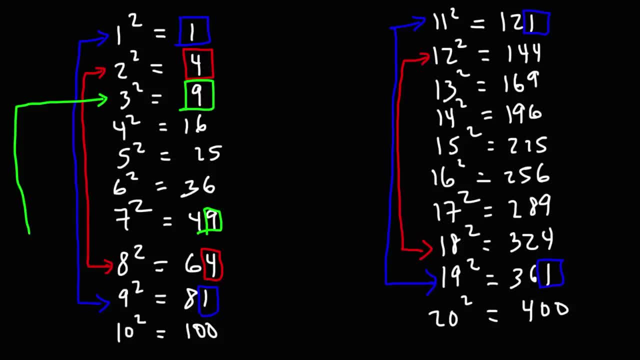 Anytime you have two numbers that end, or if you're taking a square of 3 or 7, you're going to get a number that ends with a 9.. So understanding this pattern can help us to find the square root of a very large number. 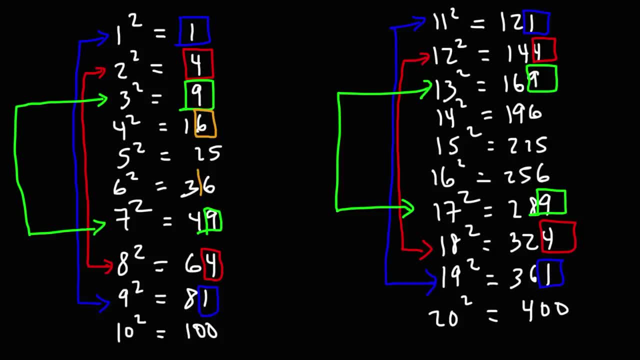 Now, anytime we square a number that ends in a 4 or a 6, the perfect square will have a unit value, a unit digit value of 6.. So 14 squared and 16 squared, their perfect squares both end up in a 6.. 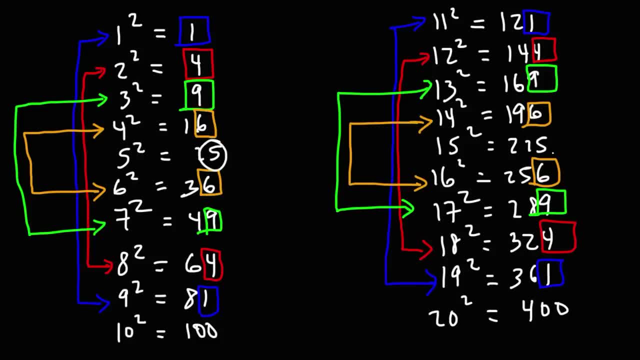 And finally, if you square a number containing 5, it will end with a 5.. And if you square a number containing a 10, it's going to end with a 0.. So those are some things that you want to keep in mind. 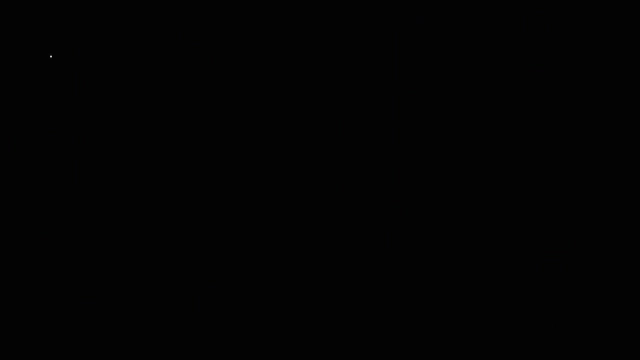 So hopefully you wrote that down, but now let's apply it to this: the square root of 1156.. So the first thing you want to do is look at the last digit, the 6.. We know that two numbers that will give us a last digit of a 6 is 4 and 6.. 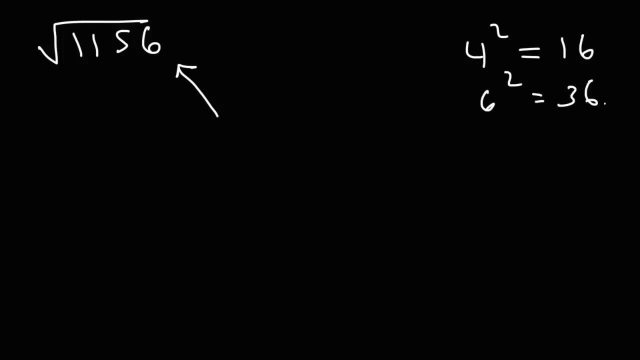 4 squared is 16, 6 squared is 36.. So the number has to end in a 4 or a 6.. Now look at the first two numbers: the square root of 11.. The square root of 11 is between the square root of 9 and the square root of 16.. 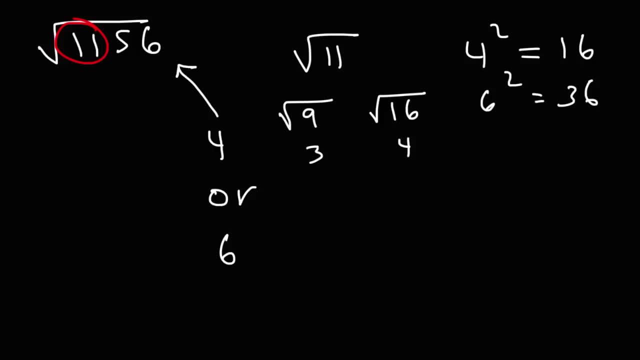 The square root of 9 is 3,. the square root of 16 is 4.. 11 is between 9 and 16, so the answer has to be between 3 and 4.. So we're going to pick the lower of the two, 3.. 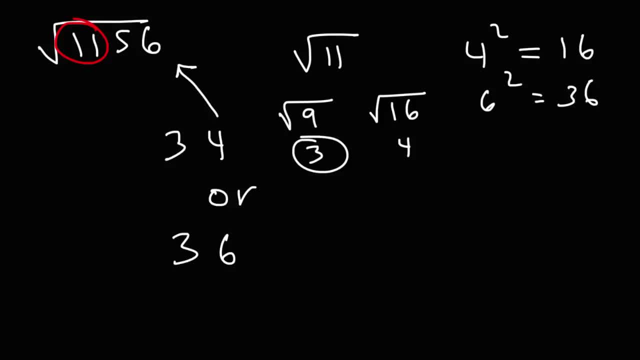 So our final answer is either 34 or 36.. The question is which one? 30 squared 3 squared is 9, so 30 squared is 900.. 40 squared 4 squared is 16, so 40 squared is 1600.. 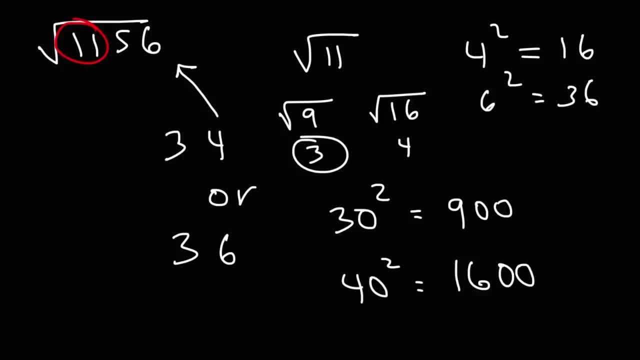 Thus the answer is going to be closer to 900.. 1156 is closer to 900 than 1600.. So we're going to pick the smaller of the two values, which is 34.. This is the answer: 34 squared is equal to 1156.. 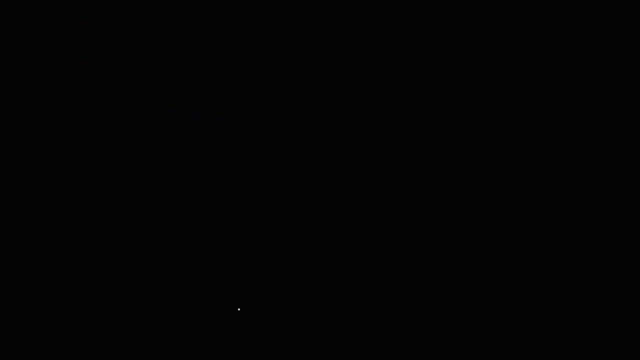 If you multiply 34 by 34, you'll get 1156.. But now let's try another example. What is the square root of 2304?? So feel free to pause the video and try this problem. So what numbers will end in a 4?? 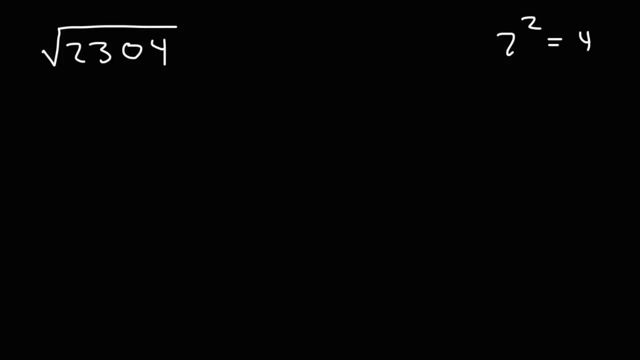 Well, we know that 2 squared is 4, and 8 squared is 64.. So the fact that we're ending with a 4 means that the last digit is either a 2 or an 8.. Now, what about the first digit? 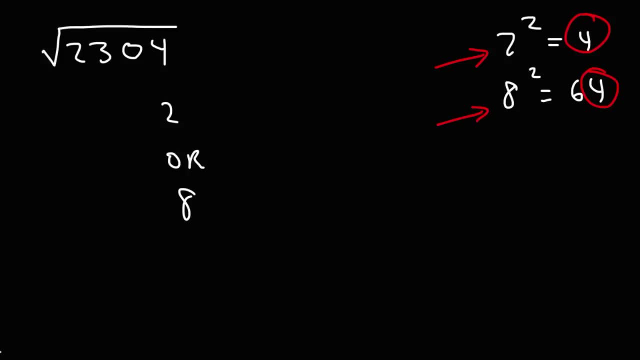 So we have the square root of 2304,, which is between the square root of 1600 and the square root of 2500.. What is the square root of 1600? That's 16 times 100.. The square root of 16 is 4, and the square root of 100 is 10,, so that's 40.. 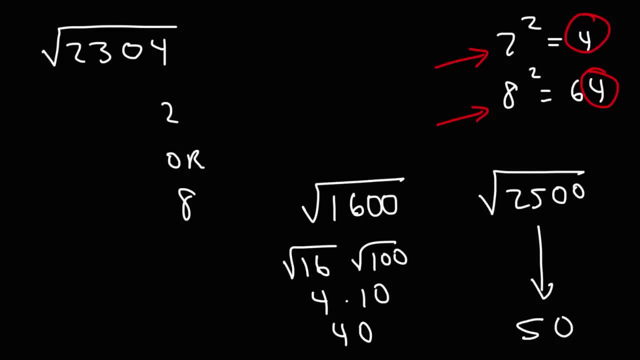 Likewise, the square root of 2500 is 50. So the answer is between 40 and 50. Well, 2304 is less than 2500, so it has to be less than 50, which means we can't use a 5.. 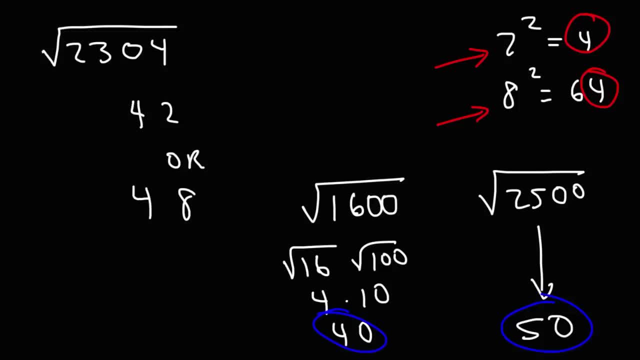 We have to use a 4 as the first digit, So the answer is either 42 or 48.. Now let's pause for a second and think about something: 2304.. This number is it closer to 1600, or is it closer to 2500?? 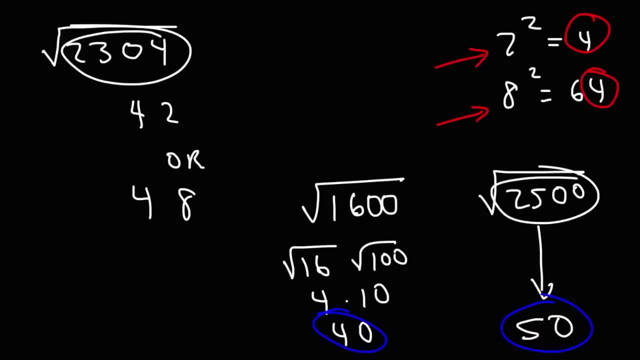 Well, 2304 is closer to 2500.. Now the answer: should it be closer to 40 or should it be closer to 50?? The final answer: should be closer to 50.. So, which one's closer? Which one's closer to 50, 42 or 48?? 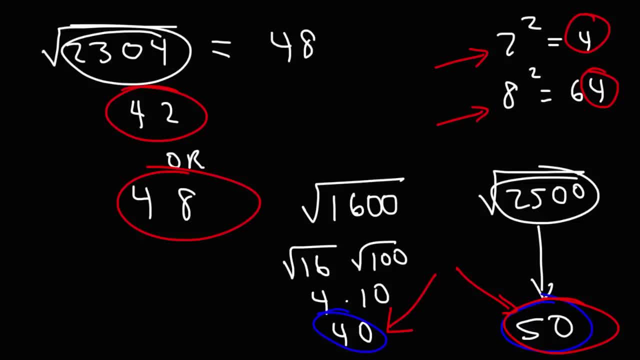 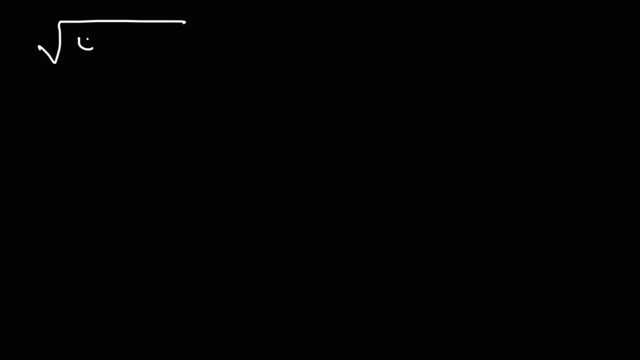 We know that it's 48. And this is the final answer. The square root of 2304 is indeed 48.. If you have a calculator, you can type it in to confirm that. So let's try another one. Let's try the square root of 4489.. 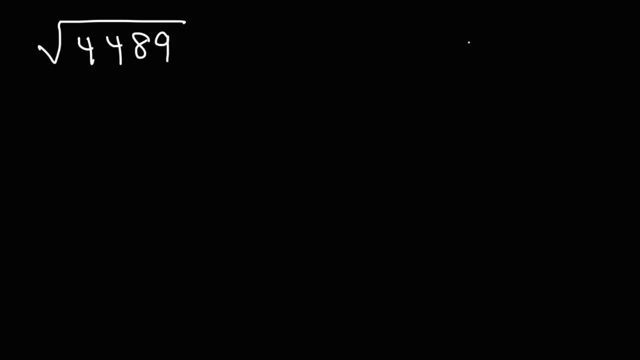 So what perfect squares end with a 9?? We know that 3 squared is 9, and 7 squared is 49. So the first digit has to be a 3 or a 7.. Now, what about the last digit? 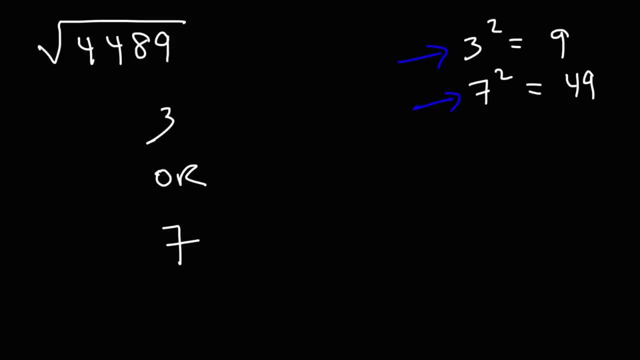 Well, let's look at the whole number: 4489.. 6 squared is 36,. 7 squared is 49. So 4489 is going to be between the square root of 3600 and the square root of 4900.. 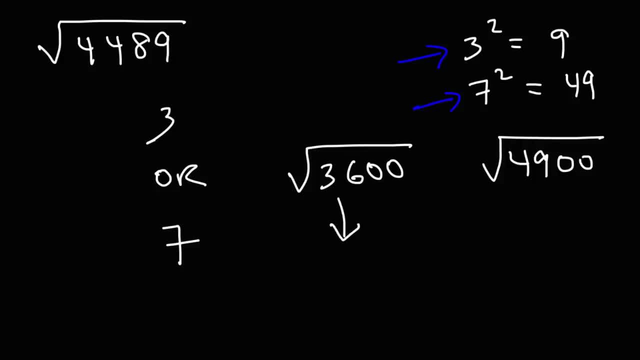 The square root of 3600,. we know that the square root of 36 is 6.. So the square root of 3600 is 60.. The square root of 4900 will be 70. So the answer is between 60 and 70.. 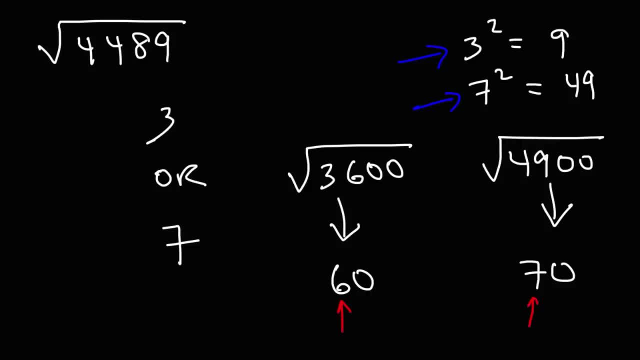 So we're going to pick the smaller of these two numbers. So the first digit is going to be a 6.. Our answer is either 6 or 7.. The question is which one is the right answer? Would you say it's 63 or 67?? 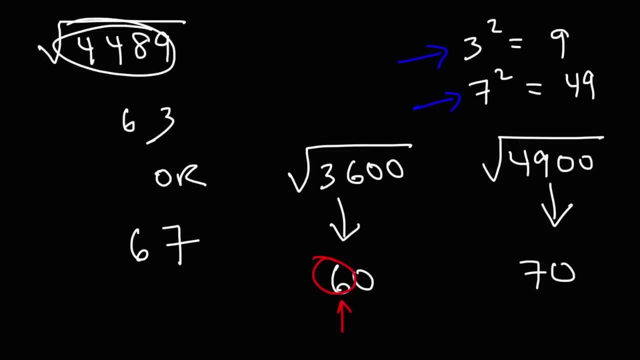 Now 4489, is that closer to 3600 or 4900?? Well, we can clearly see that 4489 is a lot closer to 4900.. So we need to pick the answer that's closer to 70.. 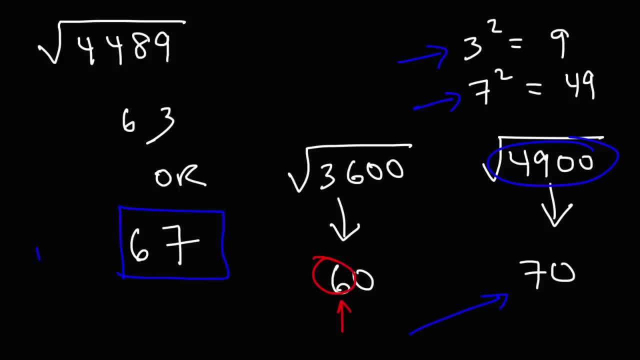 And that is going to be 67.. This is the right answer. Now let's try a harder problem. Let's try taking the square root of a five-digit number, Let's say 12,996.. Go ahead and pause the video and work on that. So what perfect squares end with a 6?? We know that. 4. 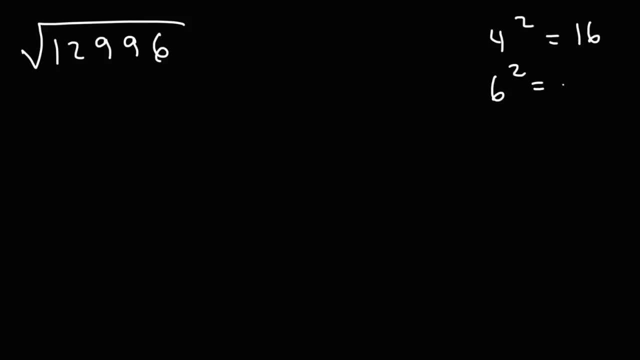 squared is 16 and 6 squared is 36.. So the last digit will end either in the 4 or in a 6.. Now we know that the square root of 10,000 is a hundred. The square root of a 12,1,000, I mean twelve thousand one hundred or 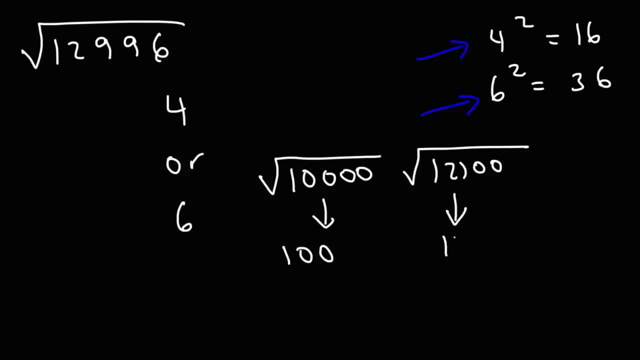 one twenty four or twelve thousand one hundred, or, informing of also a two thousand famili, and 100 is 110.. If you type in 110 squared, you're going to get 12,100.. And 12 squared is 144.. So 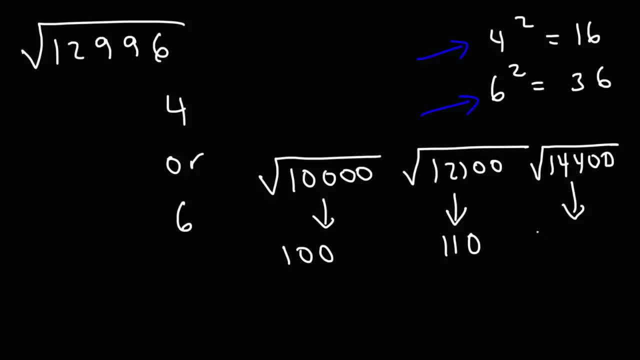 the square root of 14,400 is going to be 120.. And you could check that. All you got to do is just add a zero. Now, 12,996 is between these two numbers, So we're going to pick the smaller. 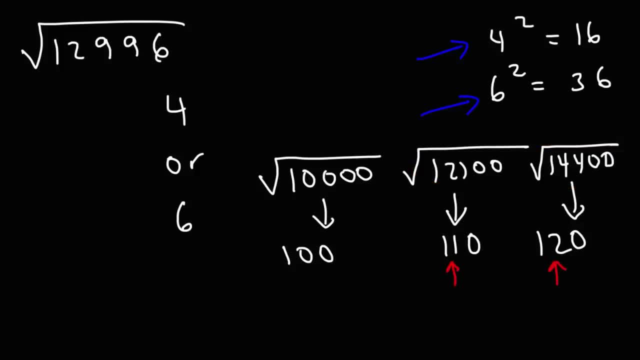 of 11 and 12, the smaller of the two numbers. So we're going to go with 11.. So the answer is either 114 or 116.. Which one is it going to be? Now? 12,996 is closer to 12,100 than it is to 14,400.